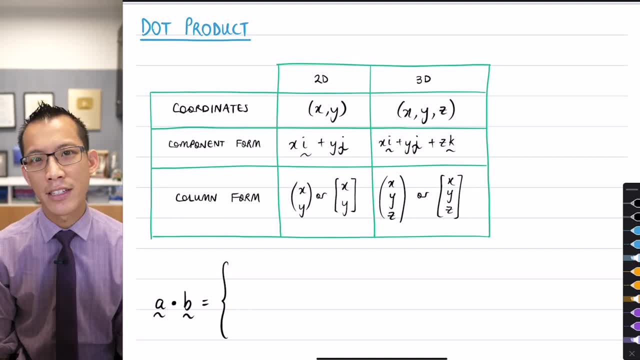 school, because that's how old I am. I learned everything that I learned about vectors when I was at university, in fact, and I remember learning about the Dot product and it was one of those many examples where I found out a formula for it and I could compute that formula. The formula is not. 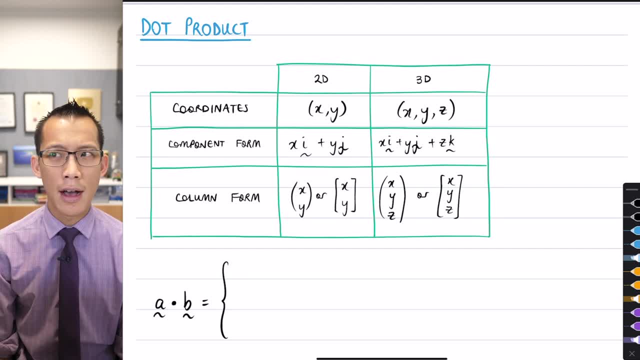 that complicated, but I never really got a sense for number one- what that formula meant, and number two, why that formula mattered. like what result or why did I care about this, right? So I'm going to try and do a bit of both. So I'm going to try and do a bit of both of those things today, which is why we're not going to go super far into this concept, because in fact, there's lots of things you can do with the Dot product and if I tried to random all into one lesson, we just wouldn't do them justice. So that's why we're just going to get a beginning into the 3D Dot product and build on some of the things you know from 2D, which is why you've got here. I don't know if you remember doing this in the first, the very first lesson that we had on 3D vectors, We created this table right and we noticed how, when you 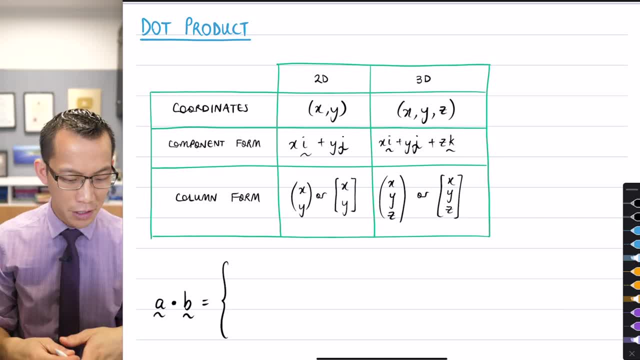 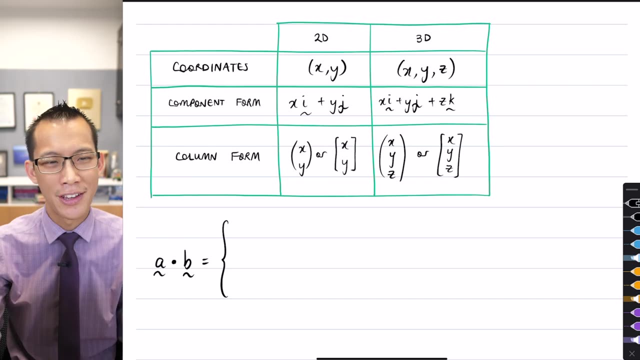 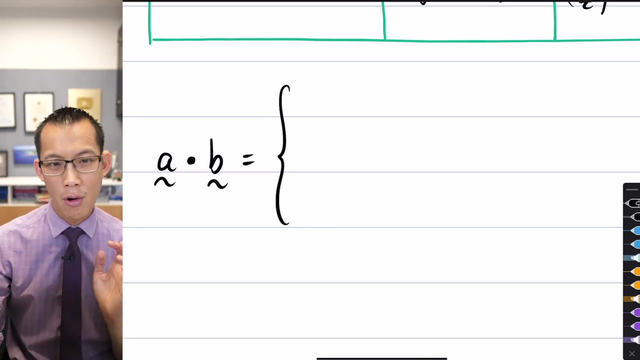 move into a three dimensional system. we take a lot of the notation and the ideas from two dimensions and we just say: go again, We did it twice before. now do it a third time, right? So I wonder if- and I am going to slightly put you on the spot here, but if you can't, if it's sort of foggy in your memory, happy to help you here- I wonder if you remember, for 2D vectors, what our definition for, or rather our formula for, the Dot product was. There were two of them, I wonder. do you remember? 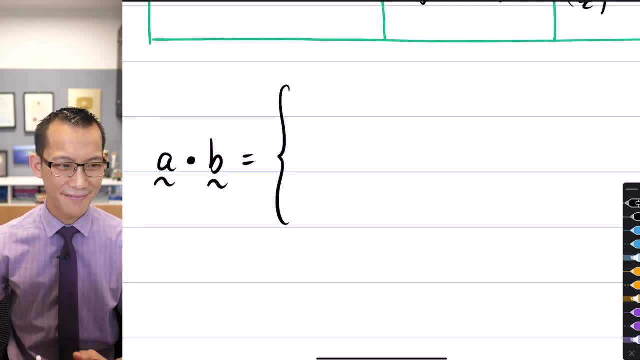 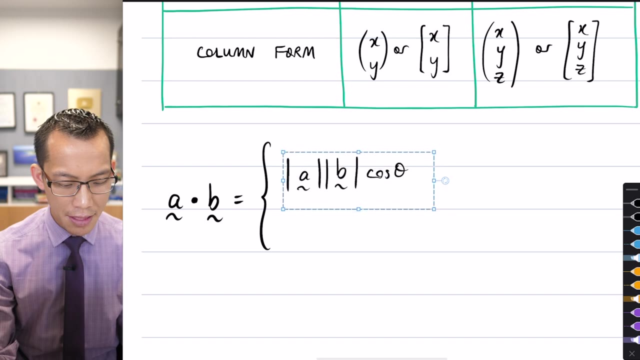 either of them. It should be absolute value of A times absolute value of B cos theta. Okay, very good. So let's just pause on this for a second, because this is- and it's worth, by the way, it's worth rewriting this. You'll see why in a moment. This is, I guess you might say, the- I would describe it as the polar formula, The polar formula, and that's because the whole idea of polar coordinates is that we can 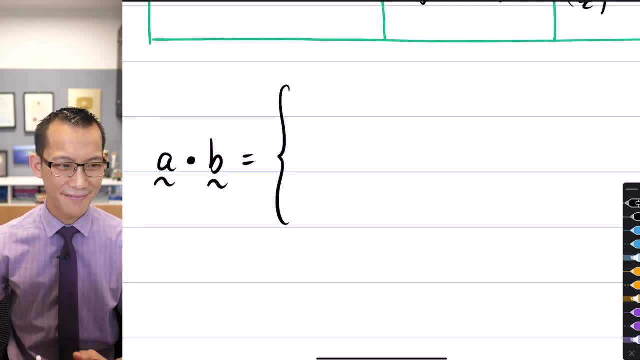 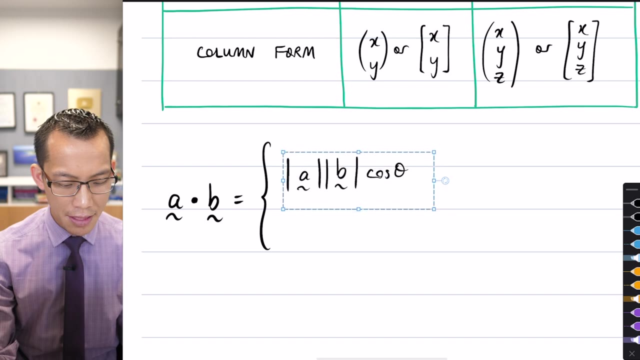 either of them. It should be absolute value of A times absolute value of B cos theta. Okay, very good. So let's just pause on this for a second, because this is- and it's worth, by the way, it's worth rewriting this. You'll see why in a moment. This is, I guess you might say, the- I would describe it as the polar formula, The polar formula, and that's because the whole idea of polar coordinates is that we can 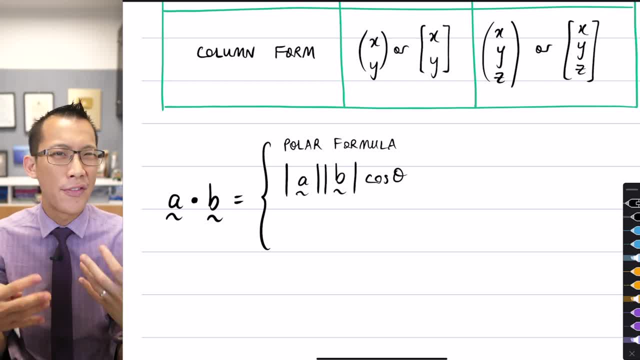 say: all right, if you've got magnitude and you've got direction, So it's a vector way of thinking, right, So you've got the, the magnitudes here, here and here, and then you've got the direction over here, Right? So what this is telling us is tell us how long A is, how long B is, and then what's the angle between the two of them, Right? And this just gives you the dot product. Okay, Fantastic. We will come back to this formula in a brief moment. But do you remember what the other one was? It had to do with the. 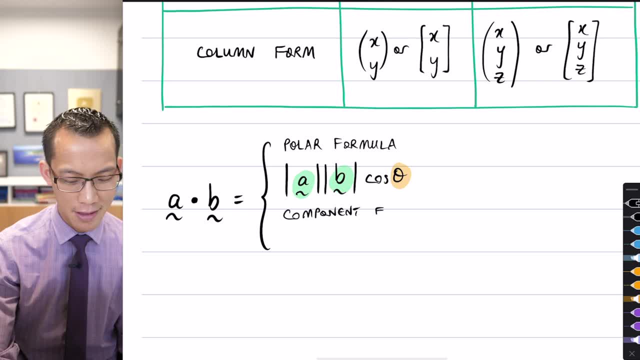 components. So I often call it component formula. Yeah, What do you remember? Say that again: X1- X2.. Okay, All right. So X1- X2.. So the X components of the first vector and then the Y components of the second, of both, of both vectors. You could call them X1- X2.. It's totally fine, I'm actually going to call them because you can see, on the left hand side my vectors are called A and B. So even though it's just a notation, 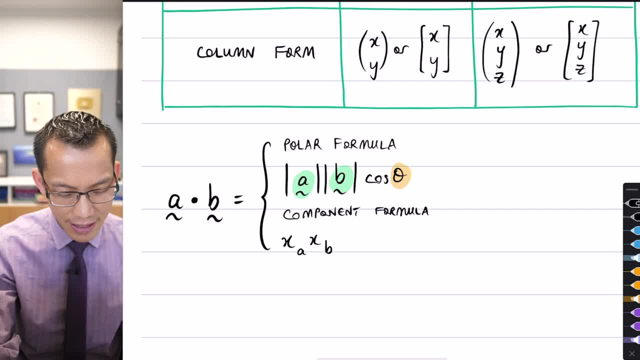 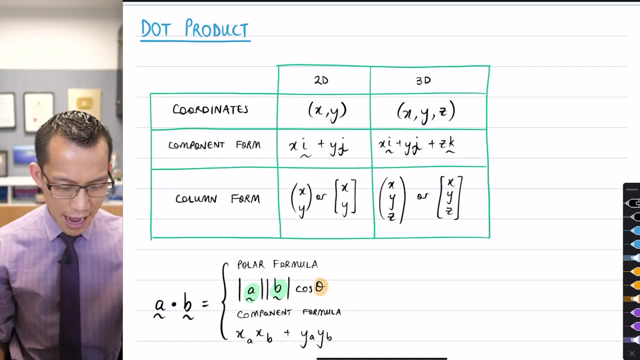 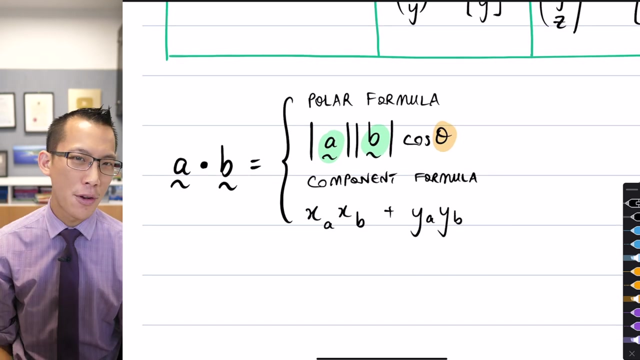 Thing. right, I'm going to call this X A, X B instead of X1, X2.. But it's not, it doesn't really make a difference, Right? And then you've got the Y components as well. Okay, Now, if you just have a look up, Right Again, this is what we looked at: extending two dimensions into three. I want you to just have a wild guess. Right, When we go into three dimensions, What would you imagine, Say, for example, the component formula is probably easier. Right, You've got the X components- monitoring- and the Y components. 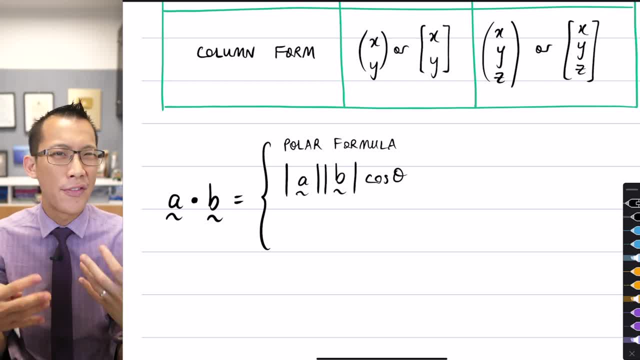 say: all right, if you've got magnitude and you've got direction, So it's a vector way of thinking, right, So you've got the, the magnitudes here, here and here, and then you've got the direction over here, Right? So what this is telling us is tell us how long A is, how long B is, and then what's the angle between the two of them, Right? And this just gives you the dot product. Okay, Fantastic. We will come back to this formula in a brief moment. But do you remember what the other one was? It had to do with the. 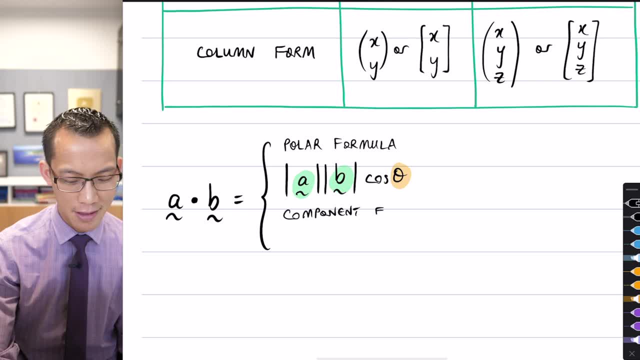 components. So I often call it component formula. Yeah, What do you remember? Say that again: X1- X2.. Okay, All right. So X1- X2.. So the X components of the first vector and then the Y components of the second, of both, of both vectors. You could call them X1- X2.. It's totally fine, I'm actually going to call them because you can see, on the left hand side my vectors are called A and B. So even though it's just a notation, 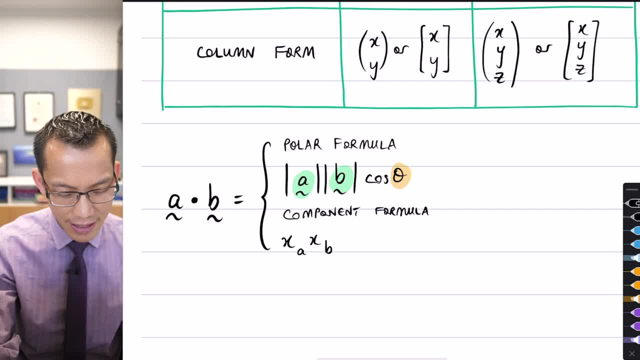 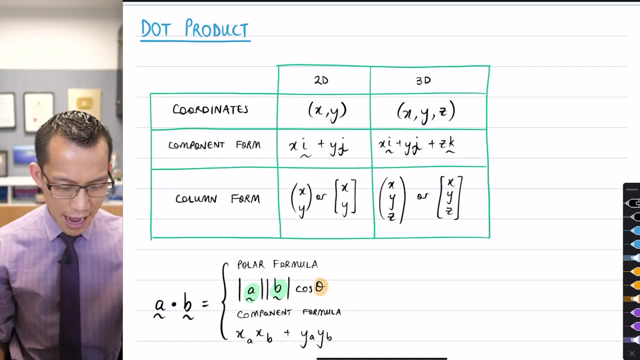 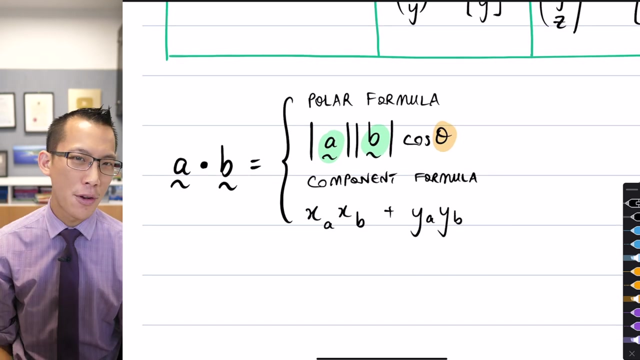 Thing. right, I'm going to call this X A, X B instead of X1, X2.. But it's not, it doesn't really make a difference, Right? And then you've got the Y components as well. Okay, Now, if you just have a look up, Right Again, this is what we looked at: extending two dimensions into three. I want you to just have a wild guess. Right, When we go into three dimensions, What would you imagine, Say, for example, the component formula is probably easier. Right, You've got the X components- monitoring- and the Y components. 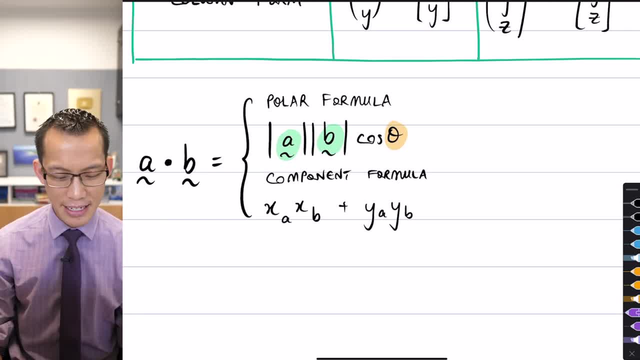 What would you imagine happens when we extend this idea into three dimensions? What would you include in addition to the X and the Y's? Yeah, Very good, So this is a fantastic guess, Right? I think it's going to be. Well, I'll just continue the pattern. Right? We multiply the X components, We multiply the Y components and added them. Why not add on the product of the Z components? Okay, Now it turns out this is exactly right, Just like 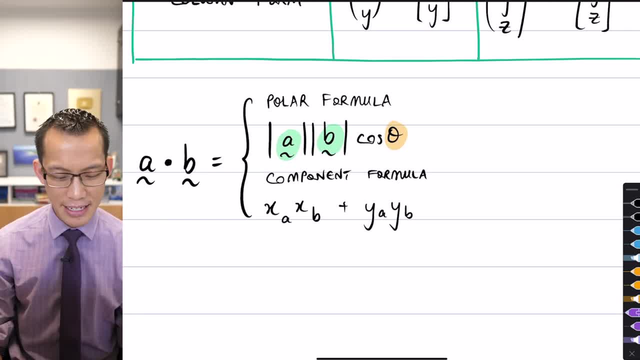 What would you imagine happens when we extend this idea into three dimensions? What would you include in addition to the X and the Y's? Yeah, Very good, So this is a fantastic guess, Right? I think it's going to be. Well, I'll just continue the pattern. Right? We multiply the X components, We multiply the Y components and added them. Why not add on the product of the Z components? Okay, Now it turns out this is exactly right, Just like 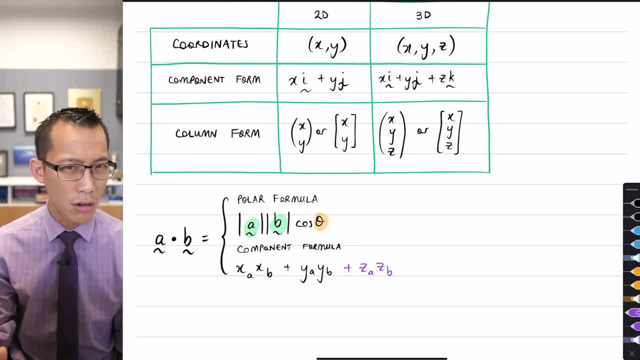 we're following the pattern. That's nice, But I actually want us to show why it is right And to understand that we actually need to look at this polar formula. I think it's it's a better definition of the dot product, because really, what you're trying to understand is: how much are A and B Like? A and B are two vectors Right, Somewhere anywhere in three dimensional space? How much are they working together with each other And how much are they working against each other, Right? That's, that's the real question. Okay, 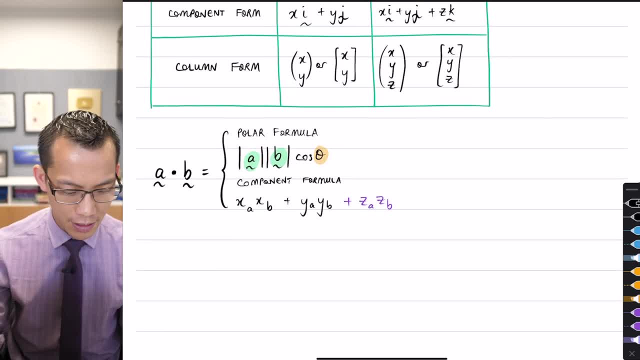 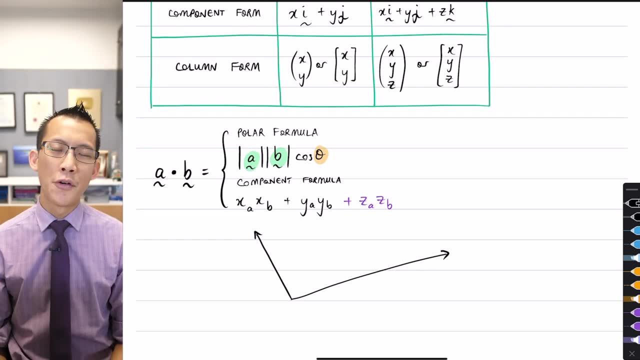 So I want us to have a picture of this, Right. So what I'm going to do is let's just draw kind of a couple of vectors, Right, Something like this, And of course, they don't necessarily actually have to be with their tails together and their heads heading out- They really could be anywhere- But because we're understanding the relationship between their magnitudes and their directions, Right, Just placing them together, tail to tail, just makes them easier to interact with, Right. So if I called this A 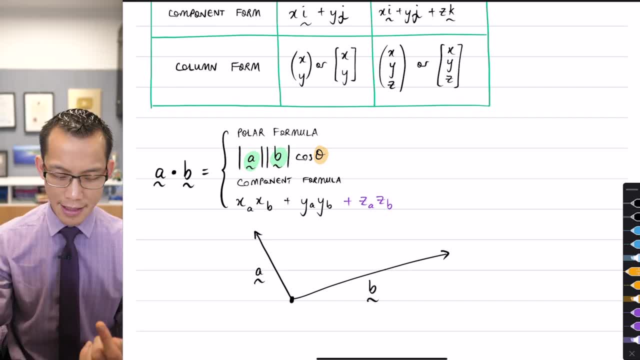 And this one B, Then that theta, that angle in between them, Is going to be in here Right Now. if we have a think about the cosine formula, This is going to be a bit strange, but not the cosine formula, The cosine graph. I'm actually going to dig a little bit into the trigonometry so you understand what's going on here and what this formula is telling you and hopefully how I can convince you that this definition makes sense of how much are they working together and how much are they working against each other. Okay, 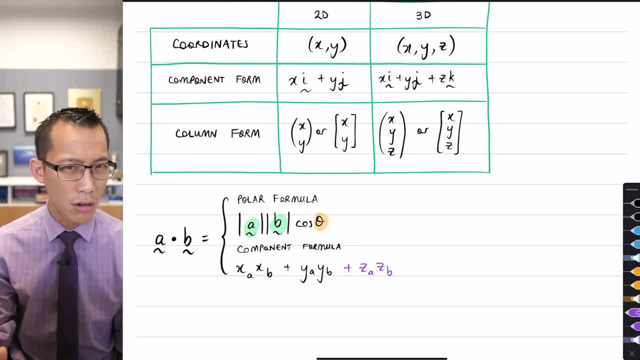 we're following the pattern. That's nice, But I actually want us to show why it is right And to understand that we actually need to look at this polar formula. I think it's it's a better definition of the dot product, because really, what you're trying to understand is: how much are A and B Like? A and B are two vectors Right, Somewhere anywhere in three dimensional space? How much are they working together with each other And how much are they working against each other, Right? That's, that's the real question. Okay, 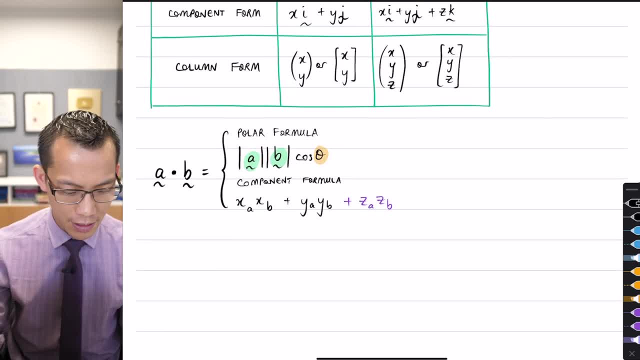 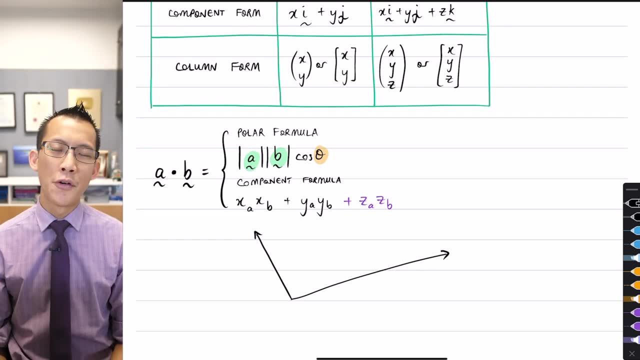 So I want us to have a picture of this, Right. So what I'm going to do is let's just draw kind of a couple of vectors, Right, Something like this, And of course, they don't necessarily actually have to be with their tails together and their heads heading out- They really could be anywhere- But because we're understanding the relationship between their magnitudes and their directions, Right, Just placing them together, tail to tail, just makes them easier to interact with, Right. So if I called this A 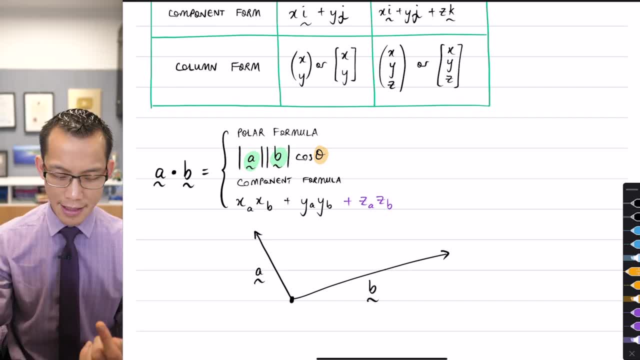 And this one B, Then that theta, that angle in between them, Is going to be in here Right Now. if we have a think about the cosine formula, This is going to be a bit strange, but not the cosine formula, The cosine graph. I'm actually going to dig a little bit into the trigonometry so you understand what's going on here and what this formula is telling you and hopefully how I can convince you that this definition makes sense of how much are they working together and how much are they working against each other. Okay, 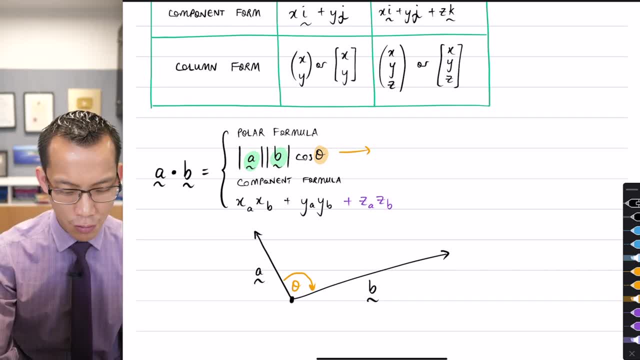 Can you do me a little favor? Near where you've, you've drawn or written this, Draw me up a small set of axes, as if we're drawing a cosine graph, because in fact, that is what we're about to do, So not with a highlighter. So let's go ahead. There we go, It only needs to be a bit rough. So what we're going to do is we're going to draw the regular cosine curve, So it looks something like this. Okay, And I want you to notice, Right. 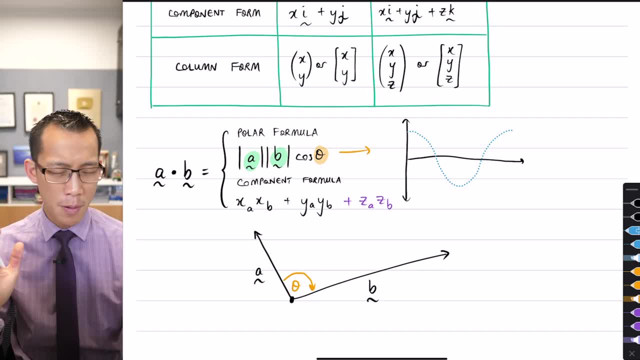 The normal cosine graph It goes from naught to two pi. I'm thinking in radians. How, By the way, how comfortable are you with radians at the moment? Is it still weird? Do you still like default back to degrees, or are you pretty comfortable? 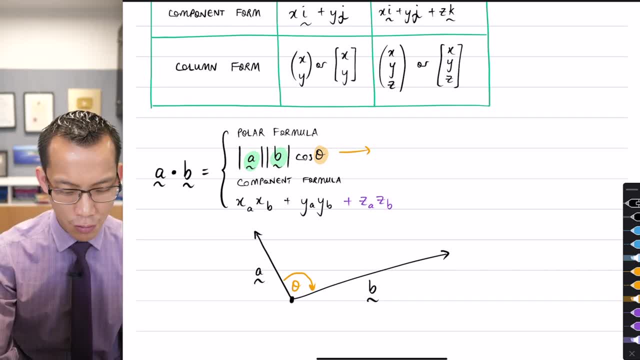 Can you do me a little favor? Near where you've, you've drawn or written this, Draw me up a small set of axes, as if we're drawing a cosine graph, because in fact, that is what we're about to do, So not with a highlighter. So let's go ahead. There we go, It only needs to be a bit rough. So what we're going to do is we're going to draw the regular cosine curve, So it looks something like this. Okay, And I want you to notice, Right. 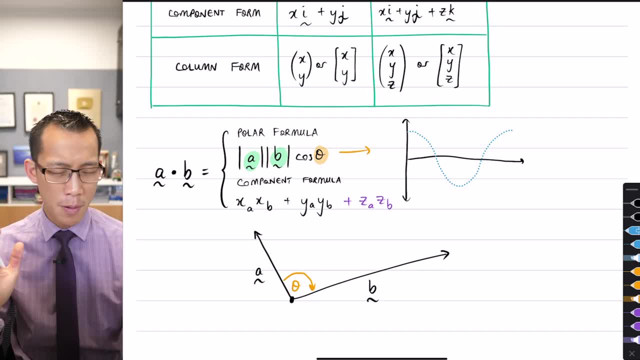 The normal cosine graph It goes from naught to two pi. I'm thinking in radians. How, By the way, how comfortable are you with radians at the moment? Is it still weird? Do you still like default back to degrees, or are you pretty comfortable? 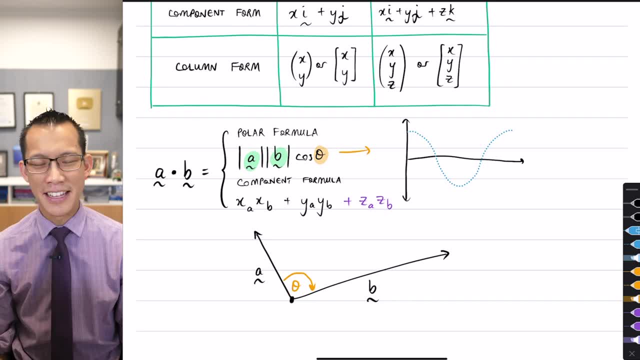 I'm comfortable with them, but I do default back to degrees. Yeah, That's, that's totally fine, It's? you know? we've been having you in degrees mode, as it were, like if your brain was a calculator. We've had you in degrees mode for, you know, 95 percent of your life. 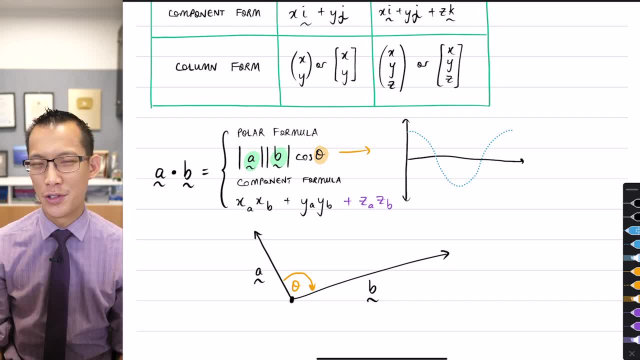 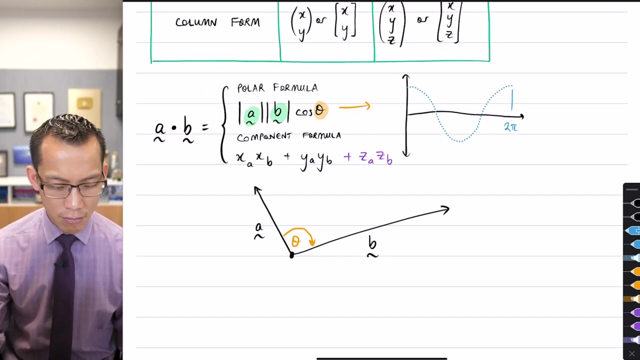 And then we're like: Hey, here's another way of doing it, And I have the good fortune of, because I've been teaching this for a long time. I've almost, like it feels, equal to me, But you will gain that familiarity with time. So what I've got here is this normal graph does end at two pi radians, 360 degrees. However, because what we're measuring here is a, an angle between two vectors, Right, You can see that if I am, you know, if I had a vector, like: let's, let's draw another one over here, Right, You don't need to draw this part, because your diagram is going to get really 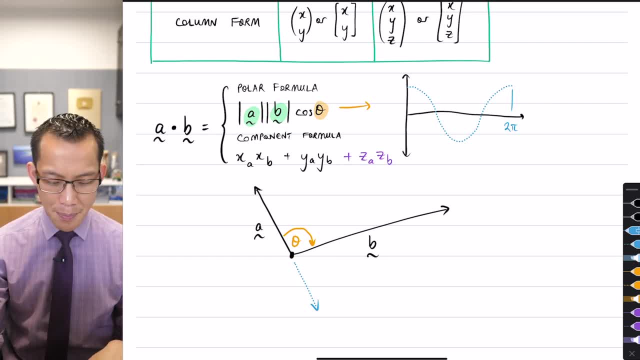 Busy really fast, Right, Can you see, if my be actually headed off in this direction, you get a theater of pi radians degree with that, like directly opposed to each other. And if I were to try and get like a larger angle, like a reflex angle, I guess, Right, If we were to, I might even take this and rotate it around. Right, If I took this and I said, OK, let's, let's spin it around this way, Right, 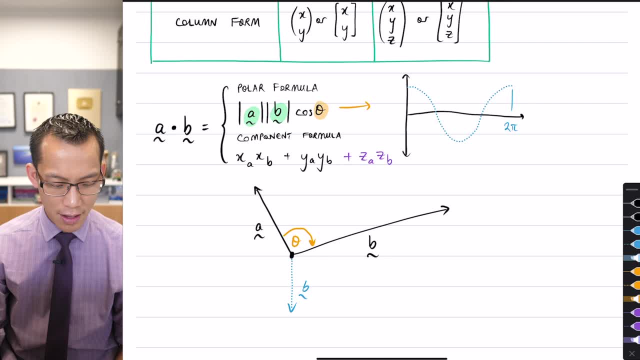 So now I have tried to increase that angle theta. what you've got is the fact that, because I'm just working out what's the angle between them, I've now got a smaller angle, this obtuse theta on the other side right, So it doesn't really like there's no reason why we 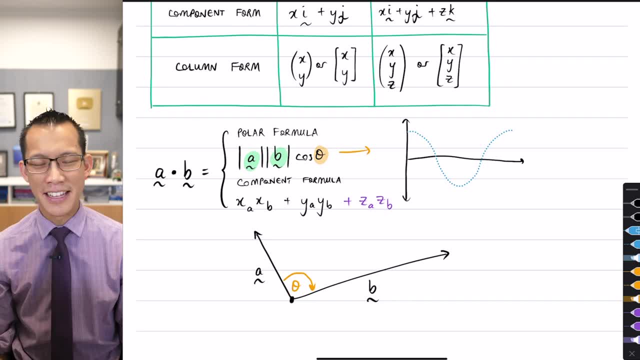 I'm comfortable with them, but I do default back to degrees. Yeah, That's, that's totally fine, It's? you know? we've been having you in degrees mode, as it were, like if your brain was a calculator. We've had you in degrees mode for, you know, 95 percent of your life. 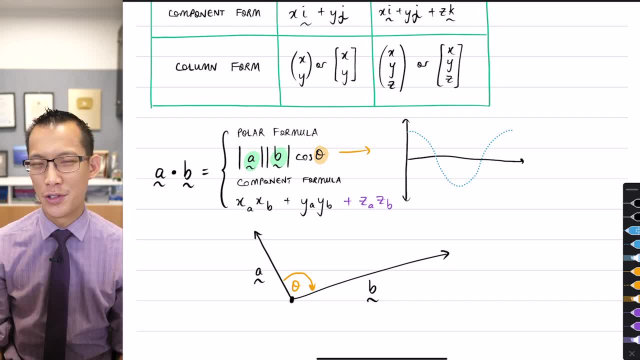 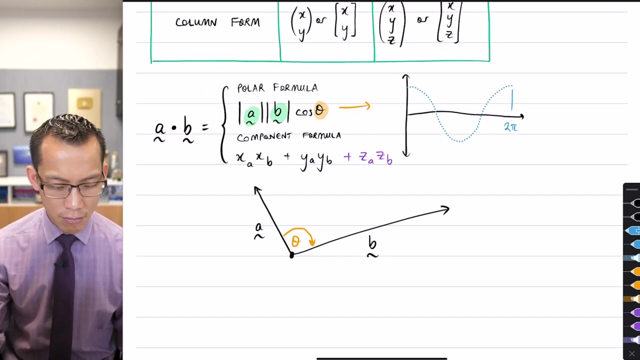 And then we're like: Hey, here's another way of doing it, And I have the good fortune of, because I've been teaching this for a long time. I've almost, like it feels, equal to me, But you will gain that familiarity with time. So what I've got here is this normal graph does end at two pi radians, 360 degrees. However, because what we're measuring here is a, an angle between two vectors, Right, You can see that if I am, you know, if I had a vector, like: let's, let's draw another one over here, Right, You don't need to draw this part, because your diagram is going to get really 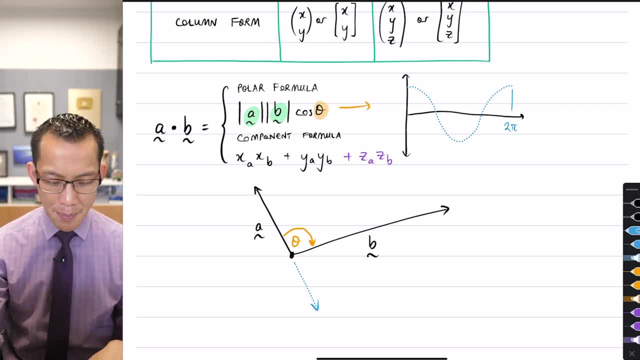 Busy really fast, Right, Can you see? if my be actually headed off in this direction, You get a theater of pi radians. do you agree with that? Like the, they're directly opposed to each other. And if I were to try and get like a larger angle, like a reflex angle, I guess, right, if we were to, I might even take this and rotate it around. right, If I took this and I said: OK, let's, let's spin it around this way, Right? 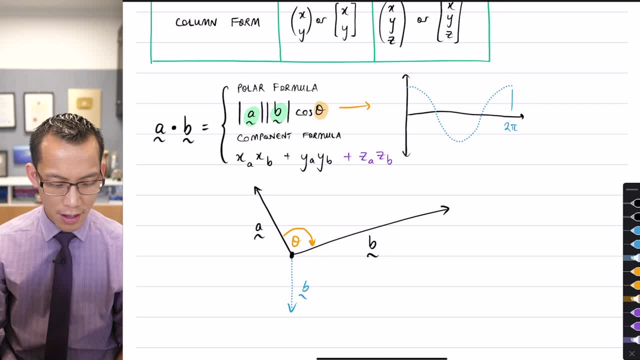 So now I've tried to increase that angle theta. what you've got is the fact that, because I'm just working out what's the angle between them, I've now got a smaller angle, this obtuse theta on the other side right, So it doesn't really like there's no reason why we 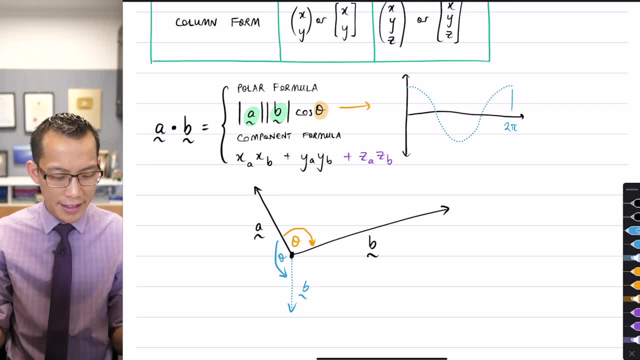 would use larger angles, like bigger than pi, if I can say the angle between the two vectors as less than pi, right? So when we think about this theta that goes in the dot product formula, we're really actually only thinking about not 0 to 2. 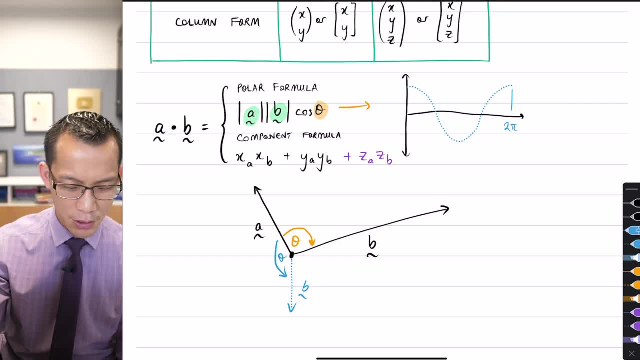 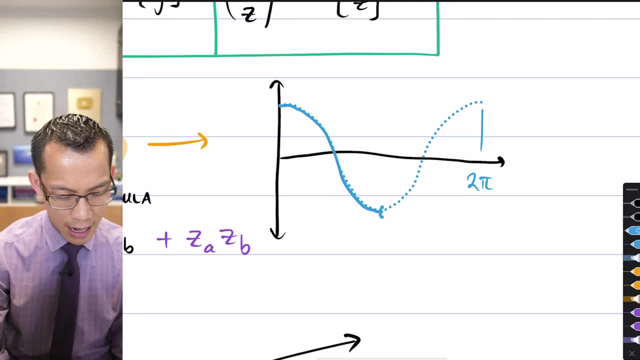 pi, but just 0 to pi. Are you content with that? So what I'm going to do is I'll zoom into this a little bit and I'm just going to emphasize this section here and I'm just going to end at pi. okay, Now you guys know we start at 0,. 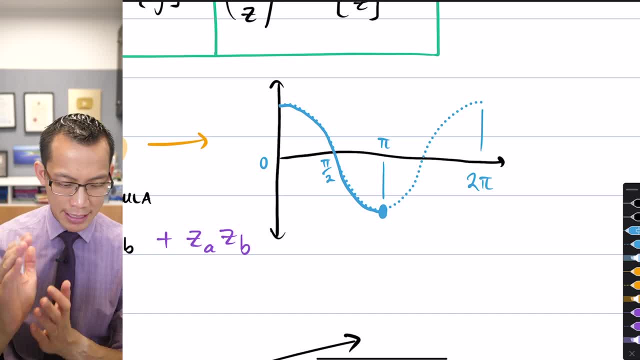 that pi on 2 is the intercept right there, and then in fact I don't really need to worry about the rest of it. so in fact I'm going to sort of get rid of all this stuff over here, just so you don't have to be confused by it. 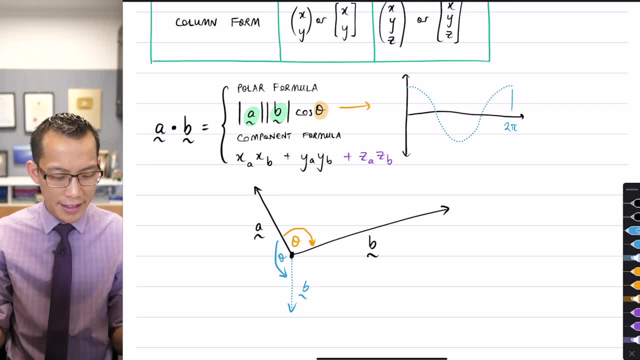 would use larger angles, like bigger than pi, if I can say the angle between the two vectors as less than pi, right? So when we think about this theta that goes in the dot product formula, we're really actually only thinking about not 0 to 2. 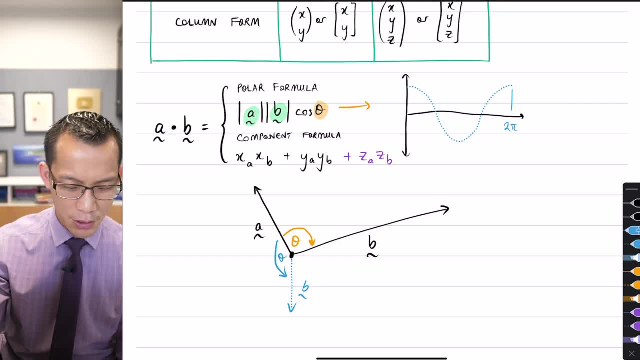 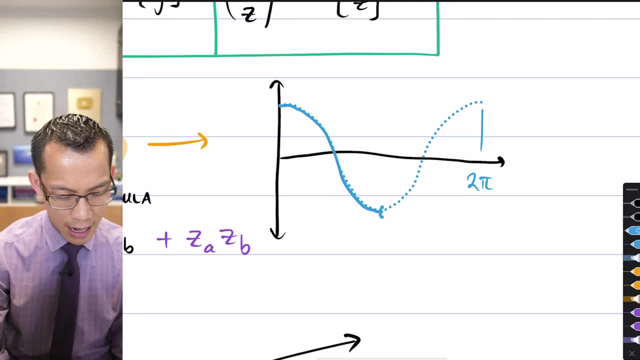 pi, but just 0 to pi. Are you content with that? So what I'm going to do is I'll zoom into this a little bit and I'm just going to emphasize this section here and I'm just going to end at pi. okay, Now you guys know we start at 0,. 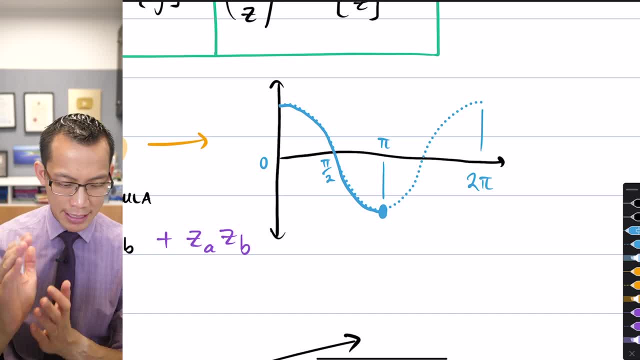 that pi on 2 is the intercept right there, and then in fact I don't really need to worry about the rest of it. so in fact I'm going to sort of get rid of all this stuff over here, just so you don't have to be confused by it. 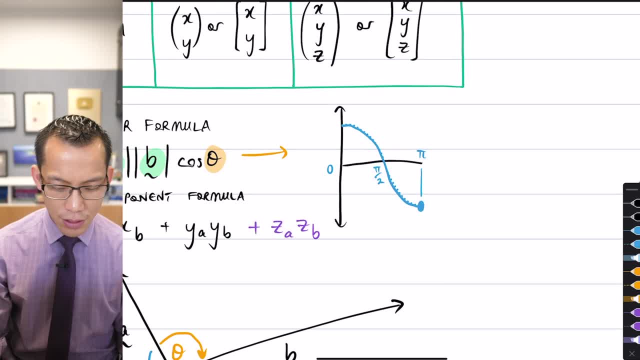 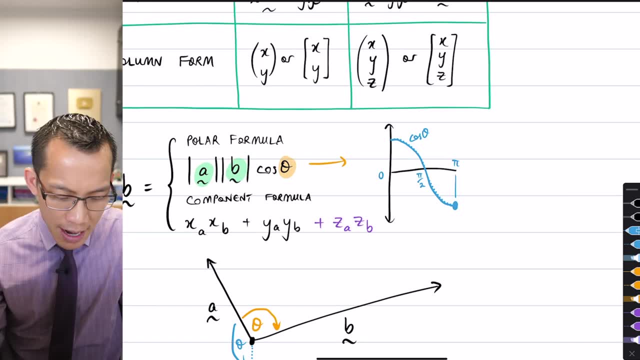 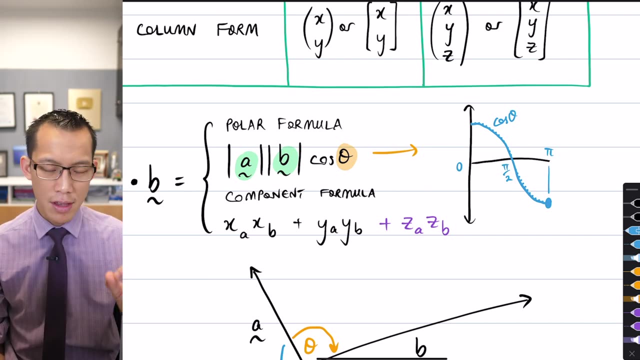 Here we go. So these are the values taken on by cos, theta in between 0 and pi. This is our domain. yeah, Now I want you to think about this. What is this telling us? okay? Well, if I've got two vectors and the angle between them is 0, right, If the 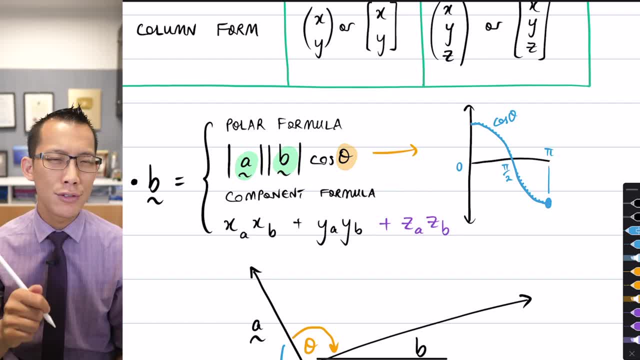 theta is 0, then when theta equals 0,, what value does cos theta take on? You can see it on the graph right: Cos of 0 is 1.. Very good, So this is the maximum. this is the highest the cosine graph goes right. 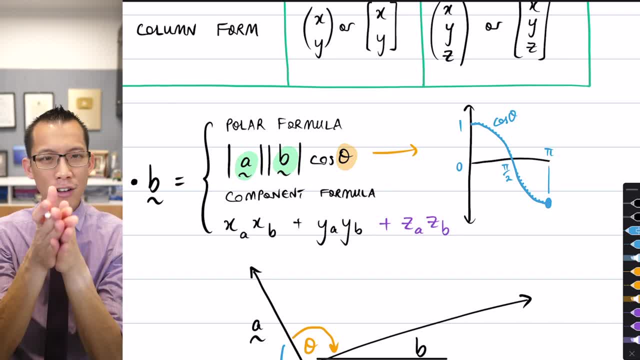 So this is kind of like all right. your angle between the two vectors is 0.. In other words, you're heading in exactly the same direction. yeah, So this is. you know. you two both like trying to get behind a car and push it in exactly the 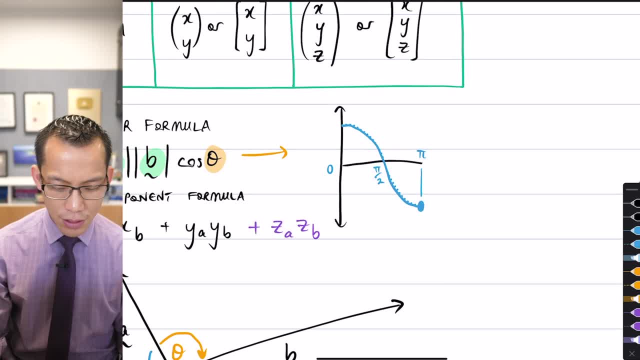 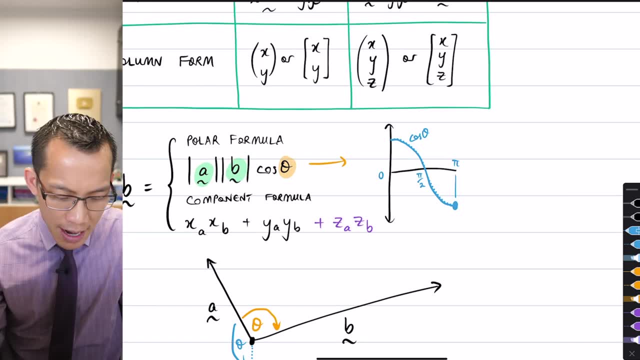 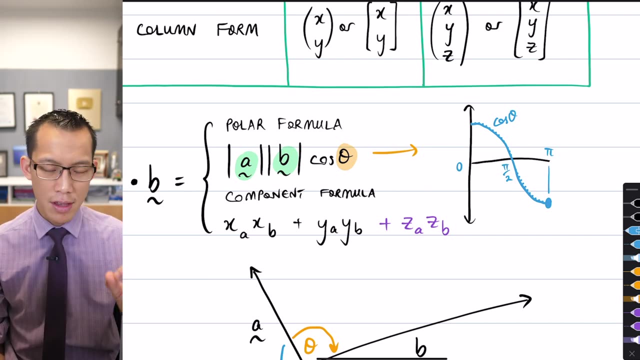 Here we go. So these are the values taken on by cos, theta in between 0 and pi. This is our domain. yeah, Now I want you to think about this. What is this telling us? okay? Well, if I've got two vectors and the angle between them is 0, right, If the 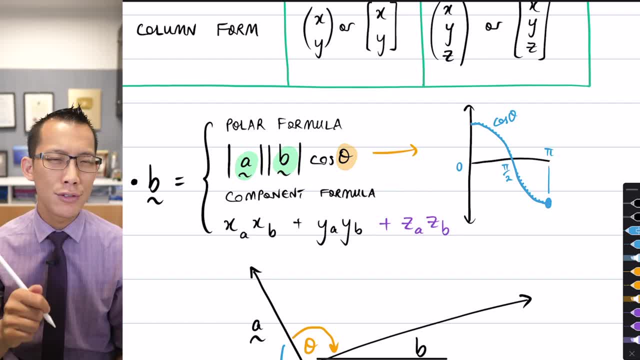 theta is 0, then when theta equals 0,, what value does cos theta take on? You can see it on the graph right: Cos of 0 is 1.. Very good, So this is the maximum—this is the highest. that cos—that the cosine graph. 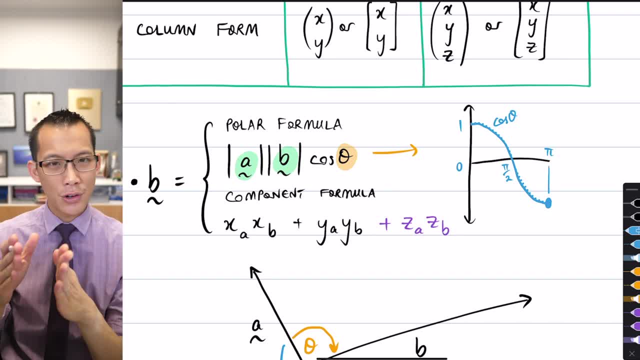 goes right. So this is kind of like. alright, your angle between the two vectors is 0. In other words, you're heading in exactly the same direction. yeah, So this is. you know. you two both like trying to get behind the car and 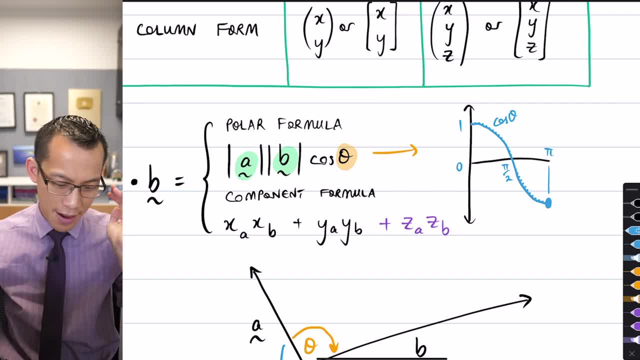 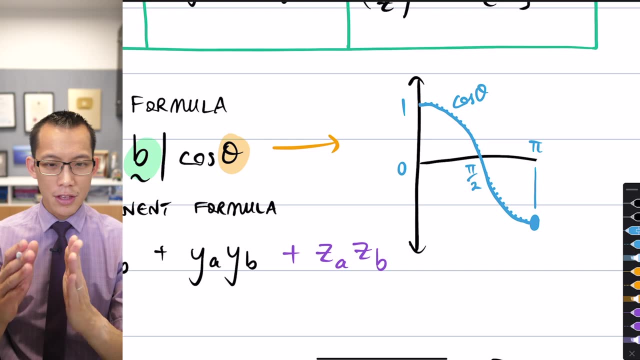 push it in exactly the same direction. so your two vectors are moving together and that's why you get that maximum value of 1, right? But then if we sort of move along the cosine graph, right, you can see as I move over to pi on 2, or as I get towards pi on 2,. your angle is no. 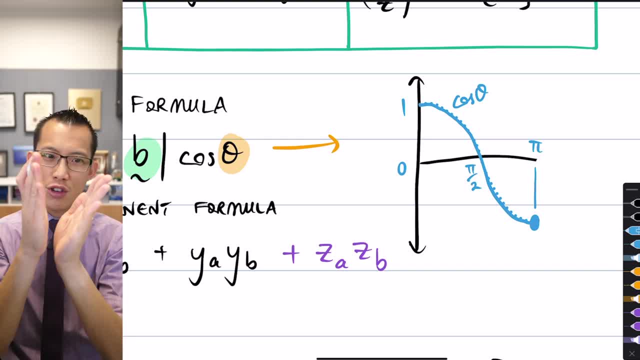 longer zero. The angle between your two vectors is kind of increasing, so you're no longer pushing in as much of the same direction. Does that make sense? The vectors are not working together as much If you get to a point where the angle theta. 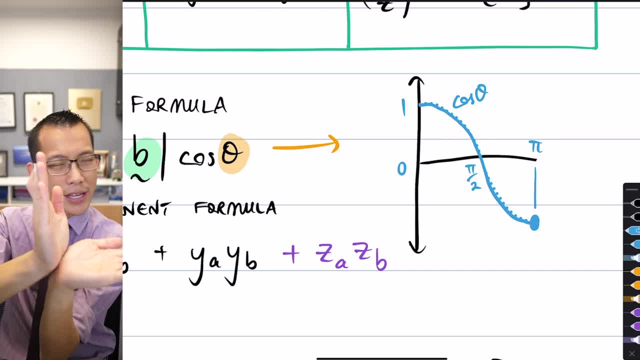 between the two vectors is pi on 2, so we would say that this is in two dimensions, we would call this perpendicular. but in three dimensions we would say: what? Start with an? o? yeah, orthogonal, all right. So these two vectors are now orthogonal. so how much are they working together with each? 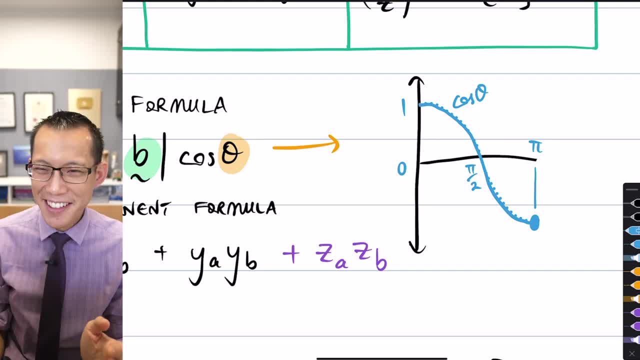 other And the answer is they're not working at all. Like if, if one of you was pushing behind the car and the other person was pushing out on the side of a car and it's going to the left or the right, it's like, hey, you're not helping. 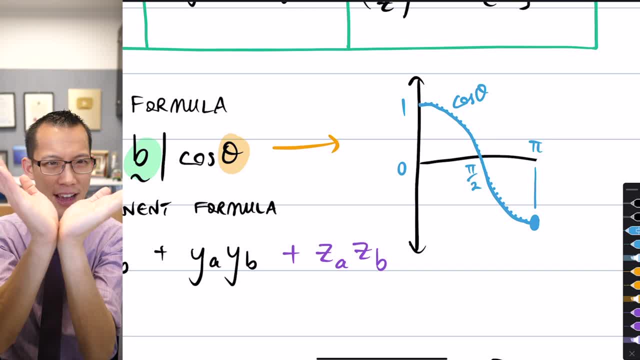 me, You're not really stopping me either, but we're not actually cooperating in any sense, and that's why cos of pi on 2 is zero, So you, you get a dot product of zero. so the vectors are not working together. yeah, and then, lastly, we 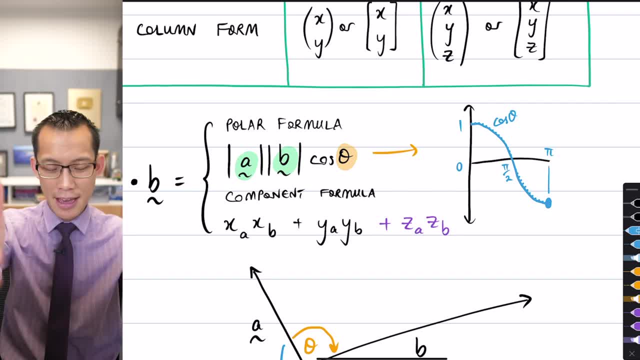 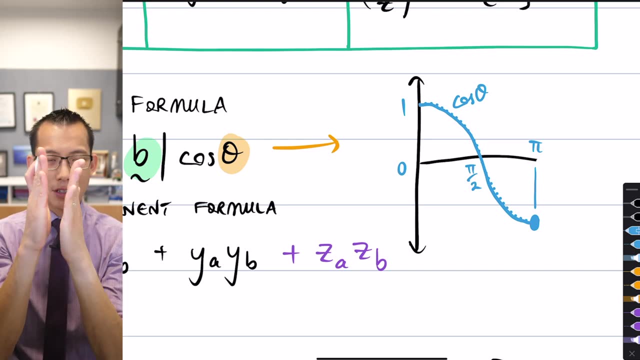 same direction. So your two vectors are moving together and that's why you get that maximum value of 1, right? But then if we sort of move along the cosine graph right, as I move over to pi on 2, or as I get towards pi on 2,, your angle is no longer 0, the angle 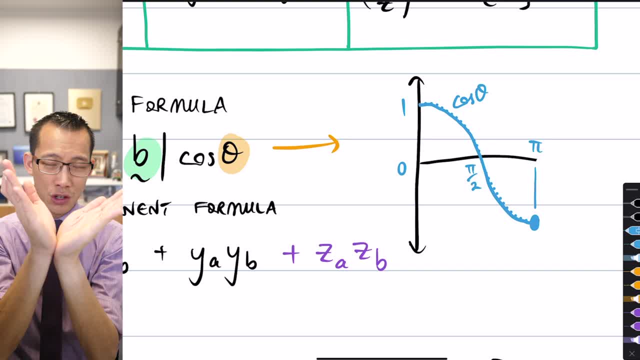 between your two vectors is kind of increasing, so you're no longer pushing in as much of the same direction. does that make sense? The vectors are not working together as much If you get to a point where the angle theta between the two vectors is pi on 2, so we 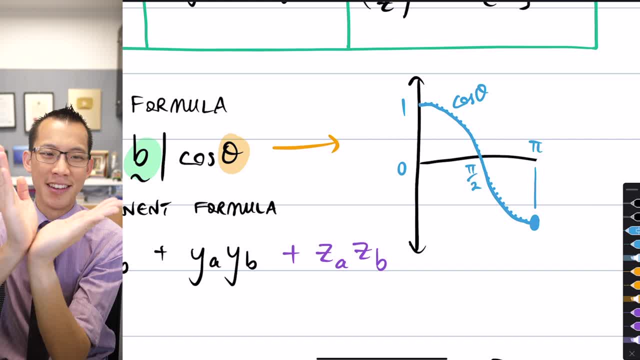 would say that this is in two dimensions, we would call this perpendicular. but in three dimensions, we would say what Starts with an O? Yeah, orthogonal, right? So these two vectors are now orthogonal. so how much are they working together with each? 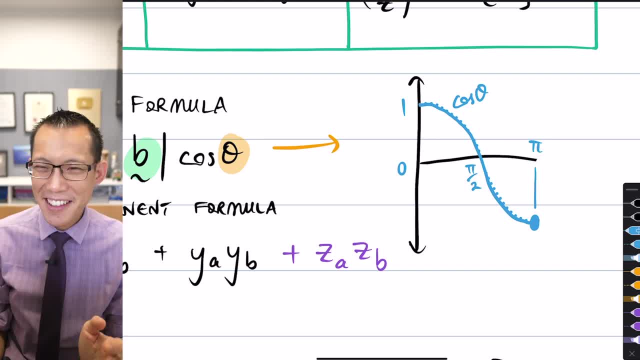 other And the answer is they're not working at all, like if one of you was pushing behind the car and the other person was pushing on the side of the car and it's going to the left or the right. it's like, hey, you're not helping me, you're not really stopping. 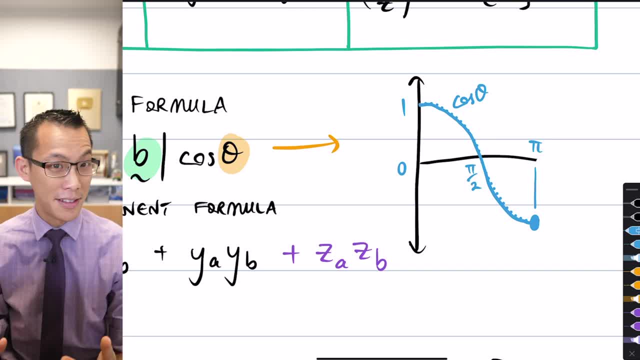 me either, but we're not actually cooperating in any sense, And that's why cos of pi on 2 is 0. So you get a dot product of 0, so the vectors are not working together, yeah, And then, lastly, we progress to this idea of past pi on 2.. 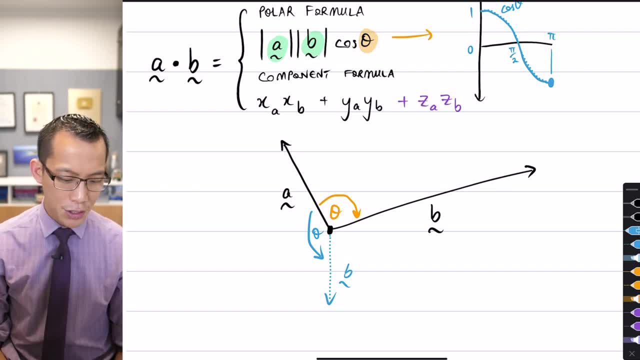 So this is actually this situation I've drawn in blue down here right. So now you've got an angle that's obtuse between them. so that's what this angle in here is: it's obtuse. So now you can picture here A and B. this is now like one of you is pushing behind the. 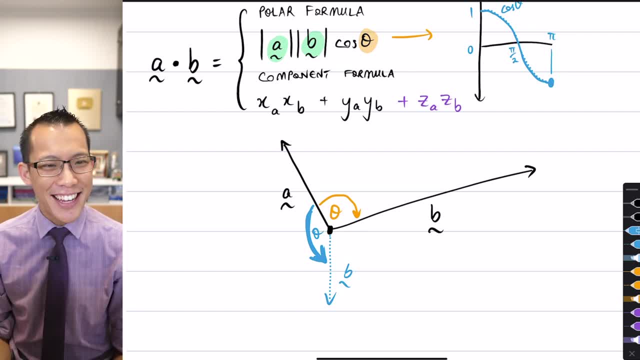 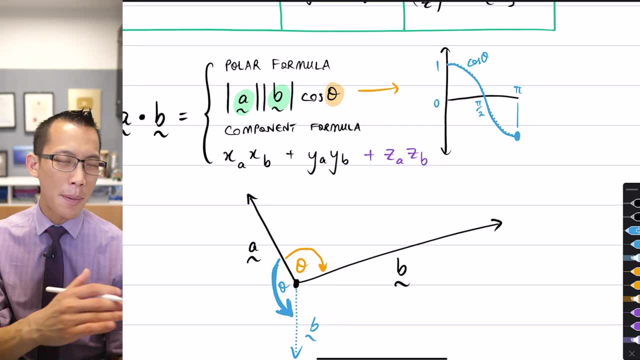 car and the other person's like on the front of the car, and you're actually pushing against each other. So what can you see about the cosine graph after you go past pi on 2, when you've got an obtuse angle between pi on 2 and pi? 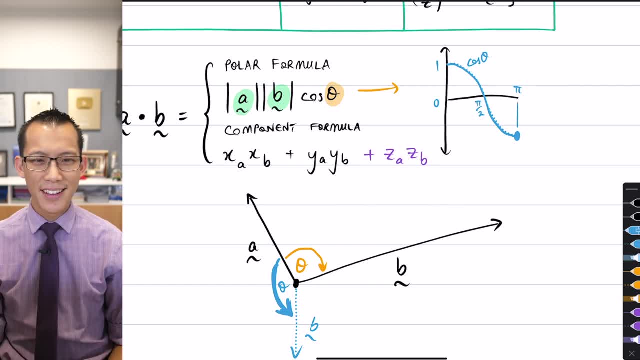 What values of cosine do you get Negative? Yeah, very good. So they're negative because they're beneath the axis, right? So this is our way of articulating that the vectors are working against each other. So this is actually quite important to say. 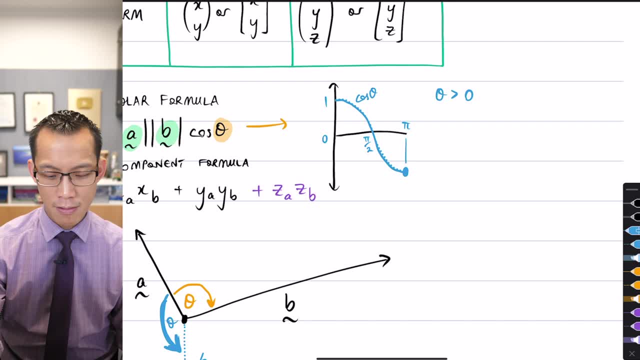 So if I said theta is greater than 0, right, what you've got is a picture kind of like this: Sorry, not theta, cos theta When cos theta is greater than 0, you've got these vectors sort of working roughly in the 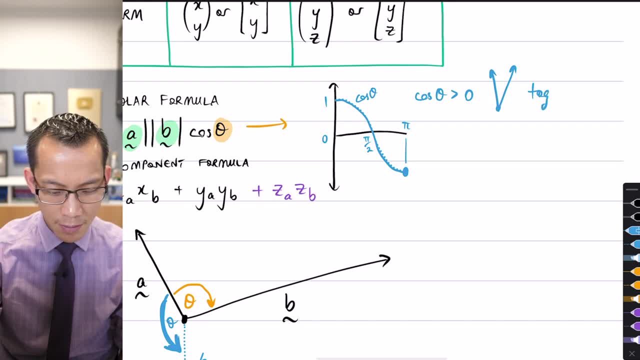 same direction, So you're working sort of together. If you've got cos theta equal to 0, right, you either have them at right angles to each other so they're orthogonal, or one of them might be the 0 vector, in which case it's. 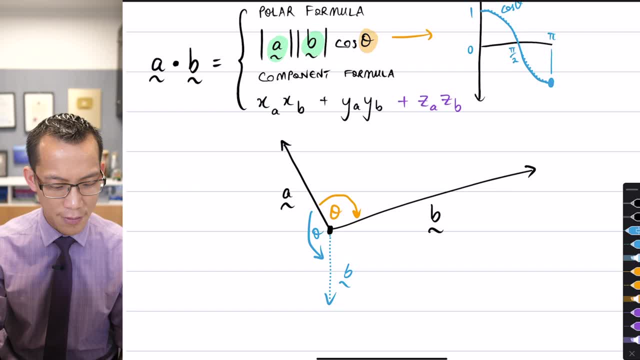 progress to this idea of pass pi on two. so this is actually this situation i've drawn in blue down here right. so now you've got an angle that's obtuse between them. so that's what. that's what this angle in here is: it's obtuse. so now you can picture here a and b. this is now like one of you. 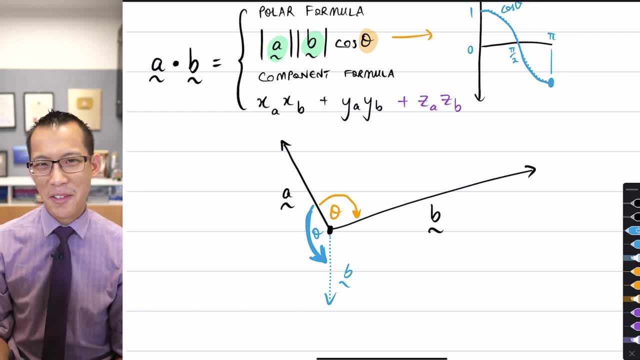 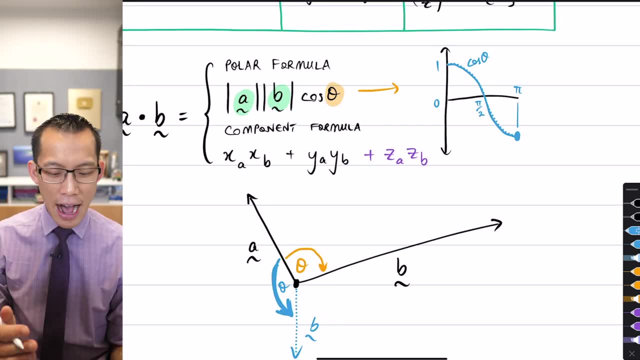 is pushing behind the car and the other person's like on the front of the car and you're actually pushing against each other. so what can you see about the cosine graph after you go past pi on two, when you've got an obtuse angle between pi on two and pi? what values of cosine do you get? 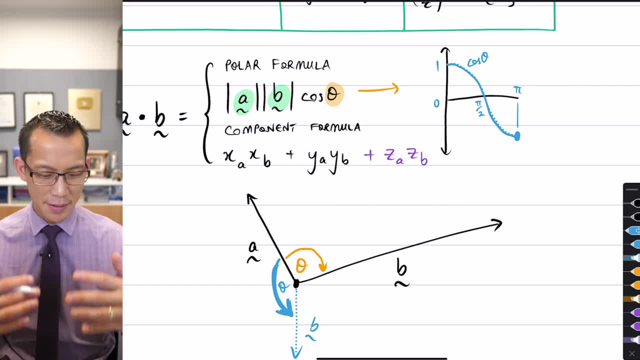 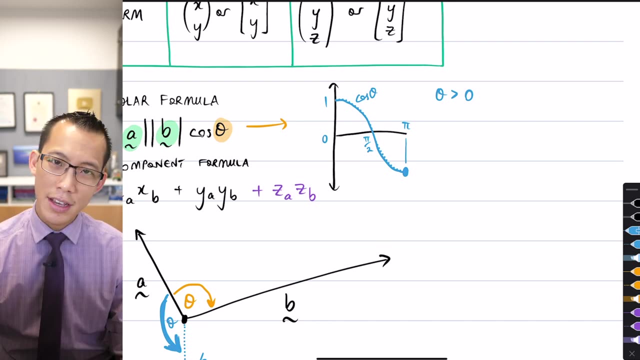 yeah, very good. so they're negative because they're beneath the axis right. so this is our way of articulating that the vectors are working against each other. so this is actually quite important to say so. if i said theta is greater than zero, right? what you've got is a is a picture kind of. 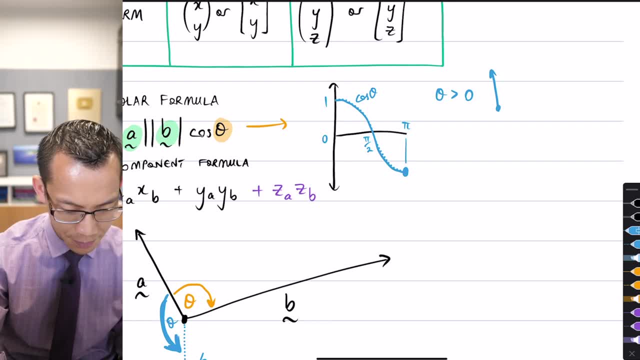 like this and you've got a vector that's working against each other. so this is actually quite like like this: sorry, not theta, um, cos theta when cos theta is greater than zero. you've got these vectors sort of working roughly in the same direction, so you're working sort of together. 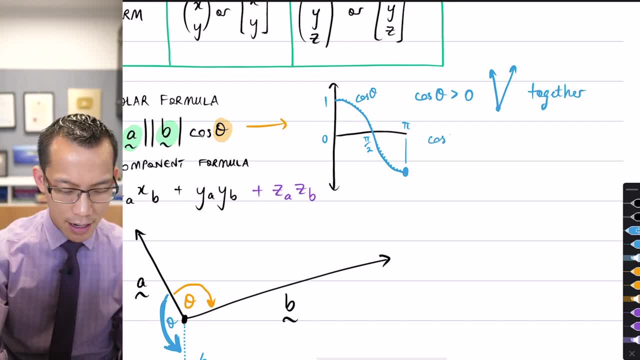 if you've got cos theta equal to zero, right, you either have them at right angles to each other, so they're orthogonal, or one of them might be the zero vector, in which case it's like one of you is just standing on the side and not pushing the car right, so you're not working together. uh, in fact it's just independent. 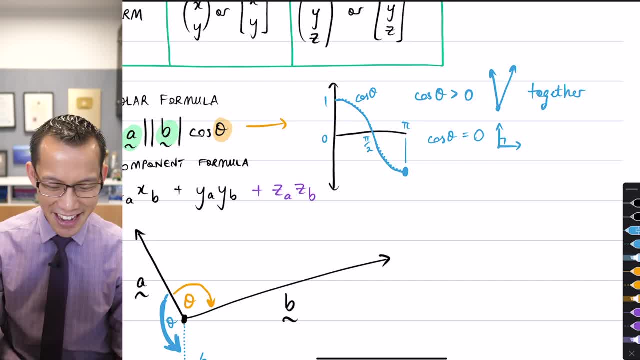 like one of you is just standing on the side and not pushing the car Right, So you're not working together. In fact, it's just independent. They're nothing really to do with each other. The two vectors aren't really contributing to each other and they're not fighting against. 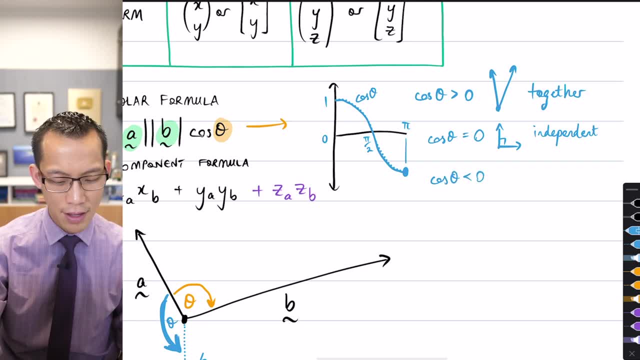 each other. And then, lastly, there's cos theta being negative. So this is where you've got a situation like this, right, Like that There's an obtuse angle or even a straight angle, right. So these are now working against each other. 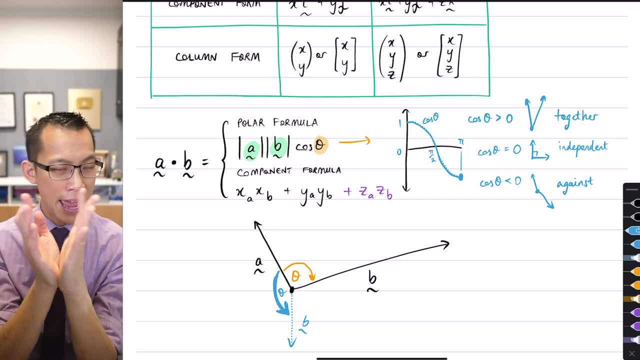 And not only do we know how much they are in relation to their angle. Right, We know their angle, but obviously if one of the vectors is very large, like the actual size of it, so you can see our magnitude of A was really big- that would increase the 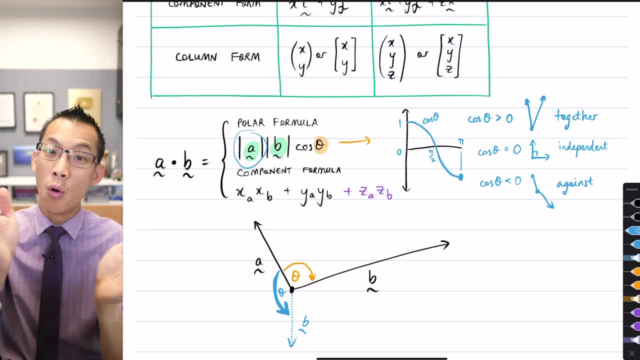 value of the dot product. So that just means they're working more and more against each other or with each other. Okay, All right. So can I just pause there? Does that make sense? Are you guys okay with that understanding? It is just so important that you get an idea in your head for what these things are doing. 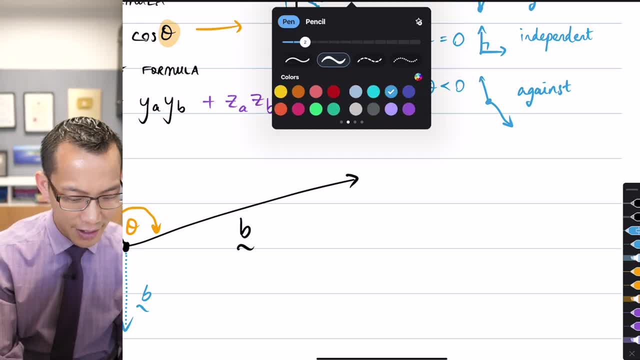 Just to give you, like another side example. you don't have to write this down, but you can if you like. You guys know the quadratic formula right. Can you actually recite it to me? X equals what's on the top. 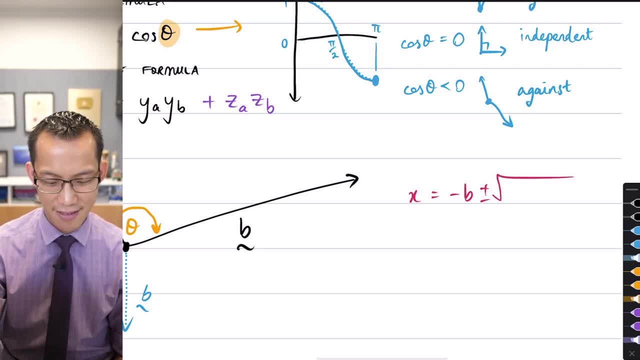 Negative B plus or minus the square root of B squared minus 4AC, all over 2A. Very good, So you've got this big mess on the numerator and then I've paused from writing 2A because I'm going to do something slightly different, right? 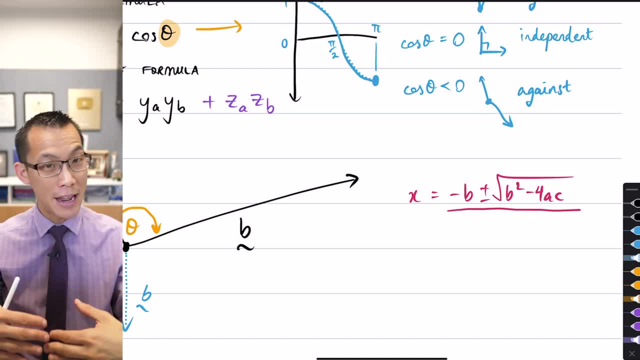 Instead of writing 2A as just one denominator down the bottom, for a reason that I'm going to hopefully make clear in a second, I'm actually going to separate this into two fractions, and I'm going to divide both of them by 2A. 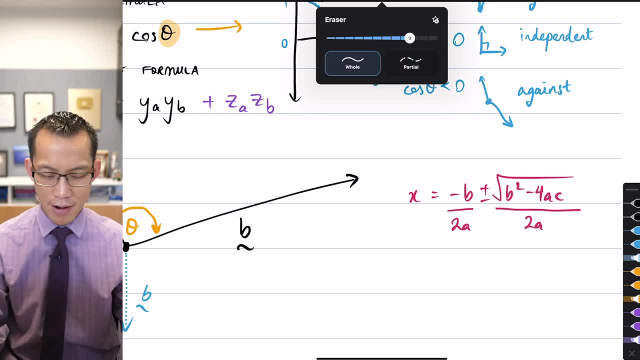 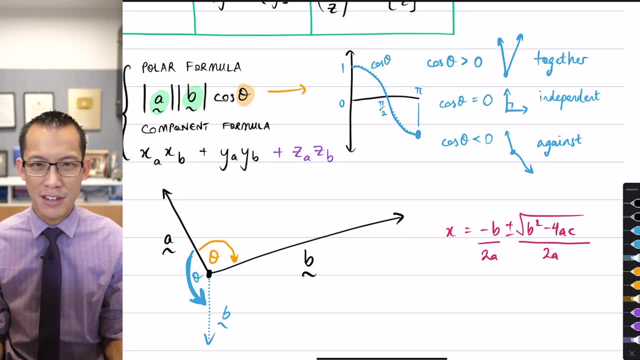 Now, the reason why I'm doing this is because I'm trying to with the dot product right? I'm trying to emphasize. I want you to know what the formula is doing and why it's doing it. Don't just see it as like: oh, there's some magnitudes and there's a cause in there, for 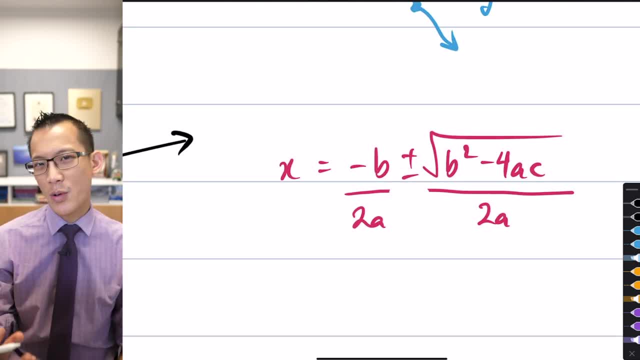 some reason right. In the same way, I want you to have a look at, like the quadratic formula, and I want you to see: do you guys recognize what is this result out the front? What is that? It's a parabola. 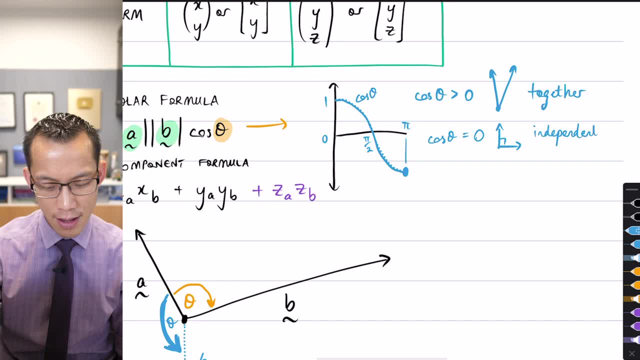 they're nothing really to do with each other. the two vectors aren't really contributing to each other and they're not fighting against each other. and then, lastly, there's cos theta being negative. so this is where you've got a situation like this right, like that. there's an obtuse angle, or even a 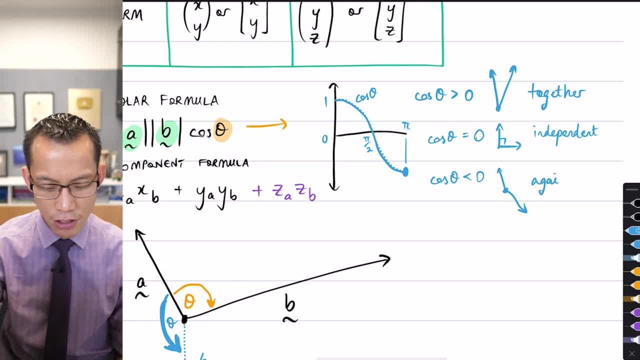 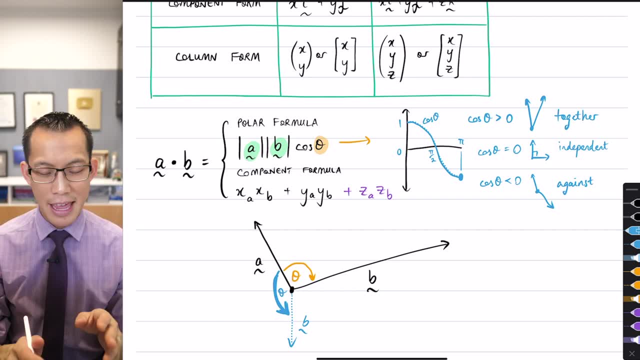 straight angle, right. so these are now working against each other, and not only do we know how much um they're working against each other, but they're also working against each other. they are in relation to their angle, but obviously if one of the um vectors is very large, that in like. 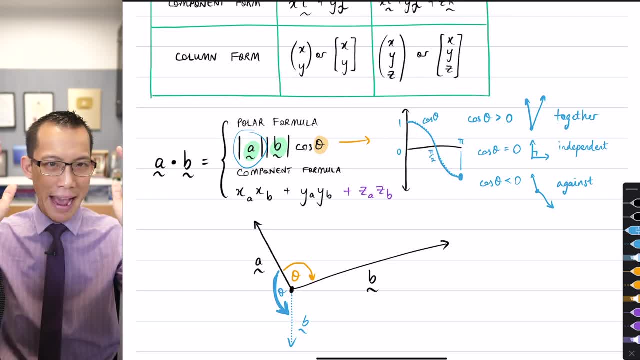 the, the actual size of it. so you can see, um, our magnitude of a was really big. um, that would increase the, the value of the dot product. so that just means they're working more and more against each other or with each other. okay, all right, so can i just pause there. does that make sense? are? 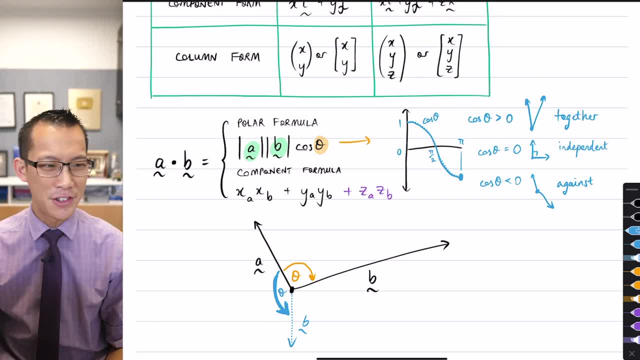 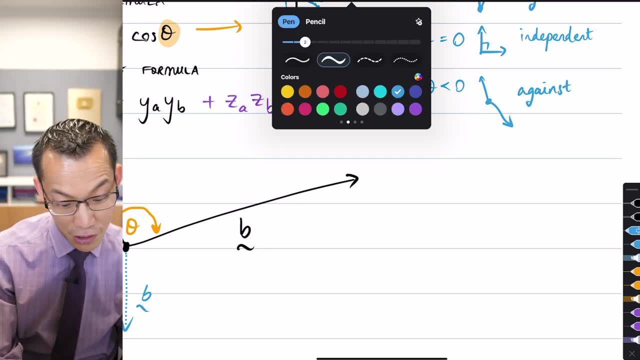 you guys okay with that understanding? um, it is just so important that you get um an idea in your head for what these things are doing. um, just to give you like another side example. you don't have to write this down, but you can if you like. um, you guys know the quadratic formula right, can you? 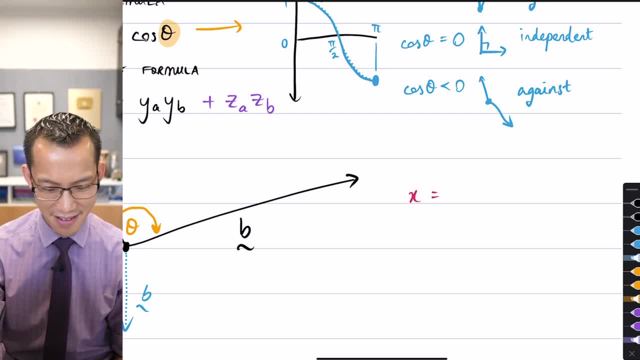 actually recite it: to me, x equals what's on the top negative, b plus or minus the square root of b squared. yep, minus 4ac. yep, all over 2a, very good. so, um, you've got these, this big mess on the numerator, and then i've paused from writing 2a because i'm going to do something slightly. 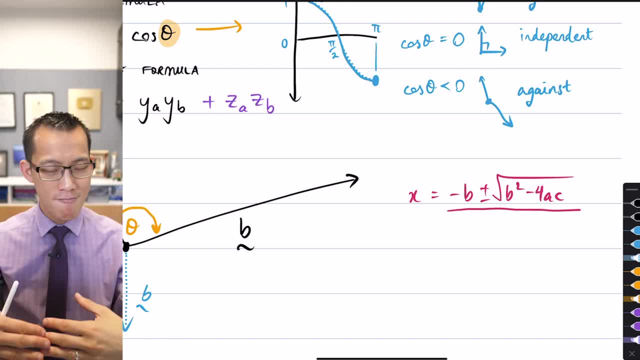 different right. instead of writing 2a as just one um denominator down the bottom, for a reason that i'm going to hopefully make clear in a second, i'm actually going to separate this into two fractions, and i'm going to divide both of them by 2a. now, the reason why i'm doing this is because 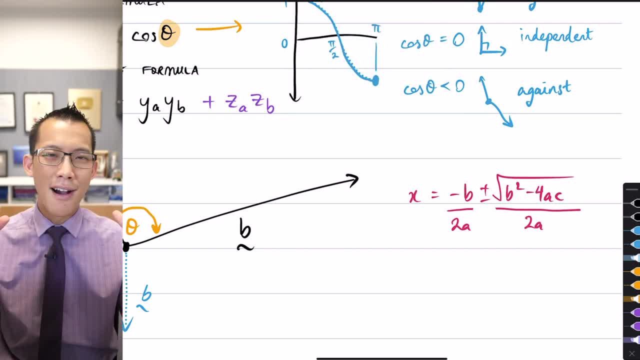 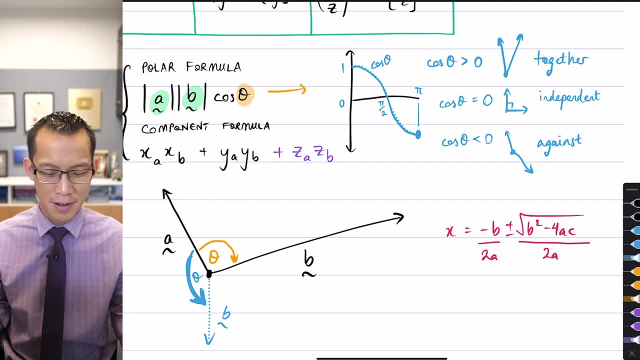 i'm trying to with the dot product, right. i'm trying to emphasize: i want you to know what the formula is doing and why it's doing it. don't just see it as like: oh, there's some magnitudes and there's a cause in there for some reason, right. in the same way, i want you to have a look at, like the: 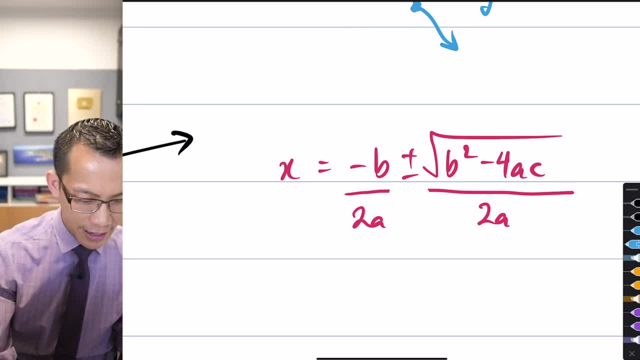 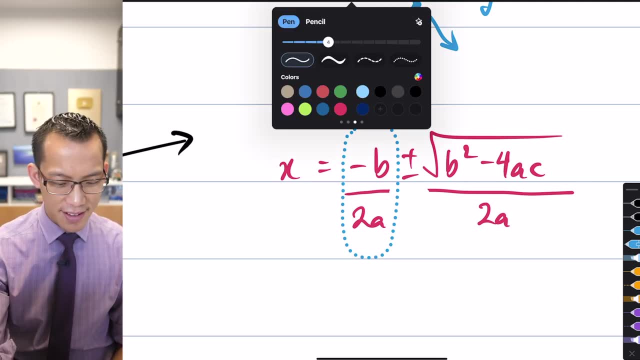 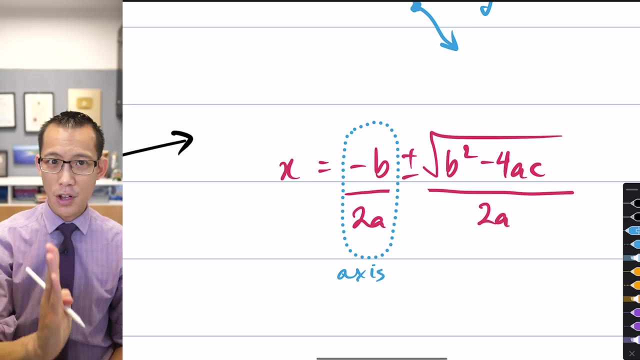 quadratic formula and i want you to see: do you guys recognize what is this um result out the front? what is this parabola? that's the it's. it's where you'll find the turning point. right, it's the axis of symmetry, it's the it's the middle of the parabola, right? and then what you do is: then you say plus, or 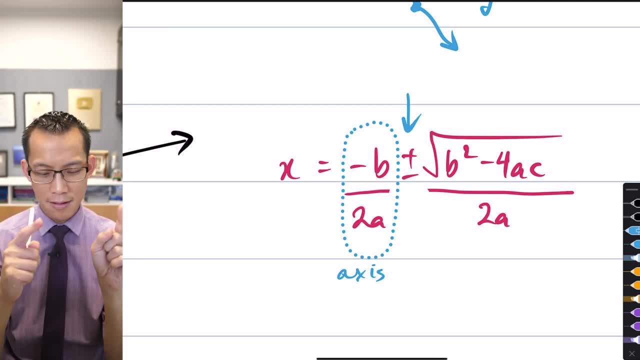 minus. so plus takes you to the right and minus takes you to the left, so you're moving on either side of it, and then what you get is is this thing here on the end which tells you where the roots are going to be right, because the roots are symmetrical around the axis of symmetry. so 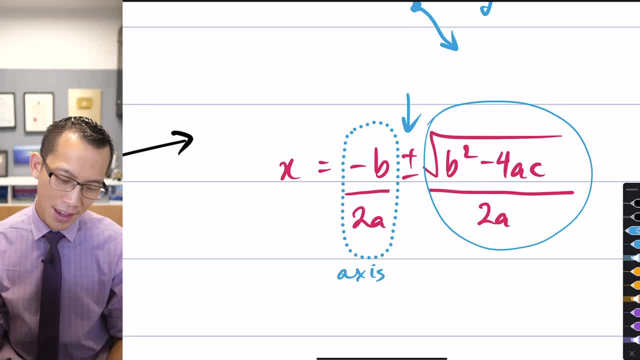 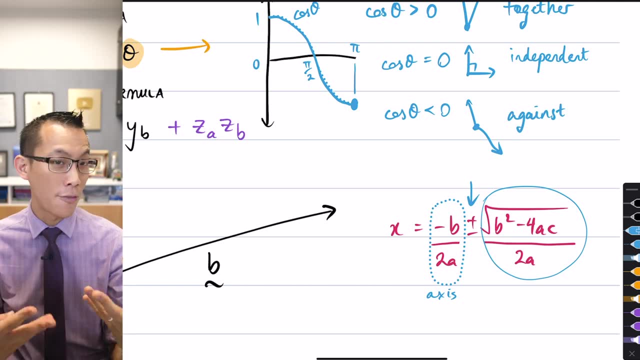 that's. that's why we call it an axis of symmetry, right? so when you look at the quadratic formula, i want you to see that it's like: oh, find the middle and then go sideways the same amount. that's what the formula is telling you. and in the same way, i want you to look at the dot product. 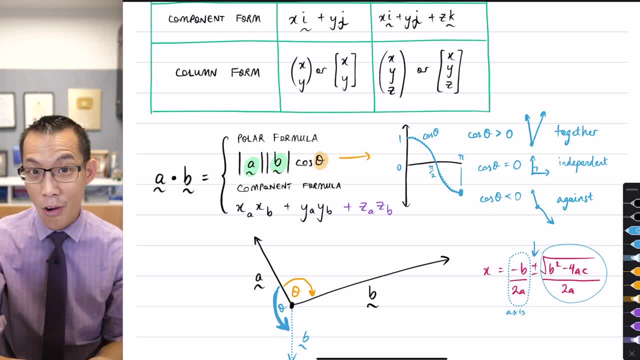 formula and i want you to say: oh, okay, it's, it's work, it's using cause, because that'll tell you whether they're working together or against each other, and then it's got those magnitudes there to work out how much they're working together or how much they're working against each other. okay, and